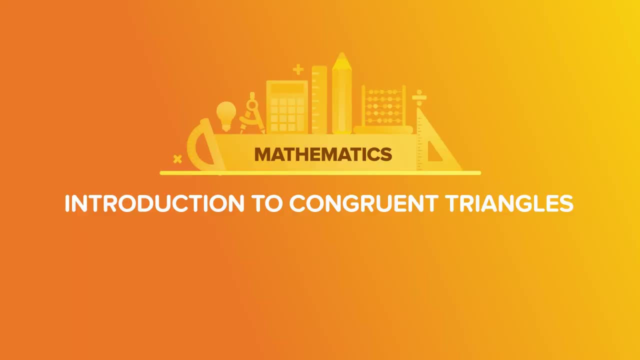 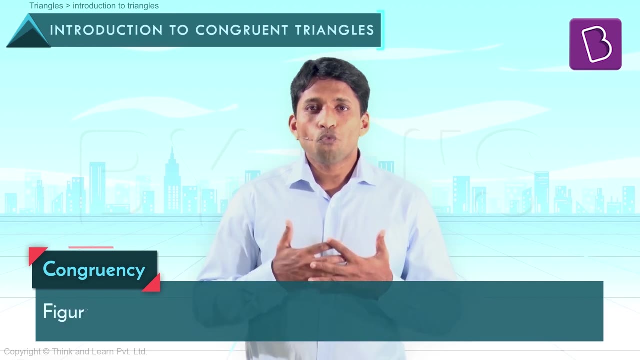 This session is about concruency and concruent triangles. So, if you ask me, what is concruency? Figures are concruent when they have the same size and same shape. So it's a very basic concept and it can never be complex. In simple words, concruency can be taken as equality. 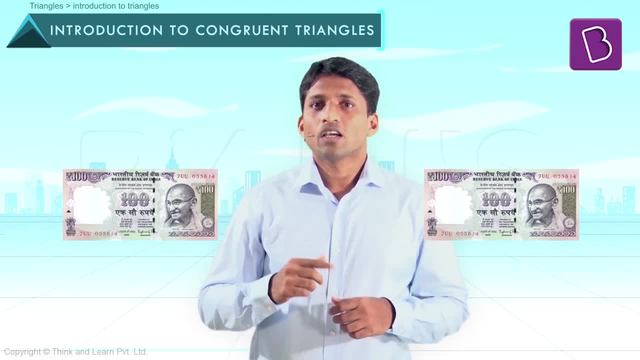 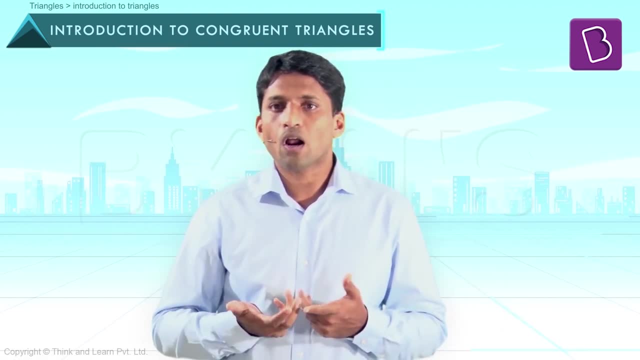 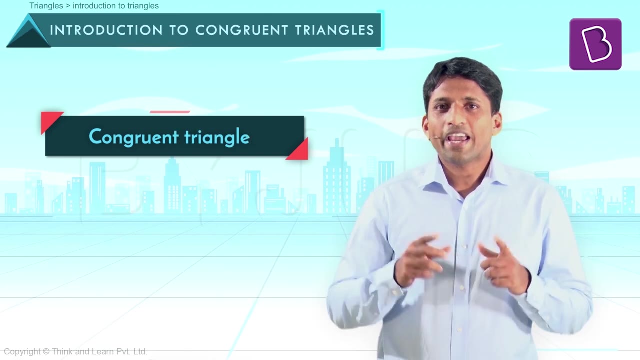 Look at these hundred rupee notes. Are they concruent? Yes, they are, because they have the same shape and the same size, Like this. if you look around, you'll come across hundreds of examples of concruency in real life. Two triangles are concruent if the sides and angles of one. 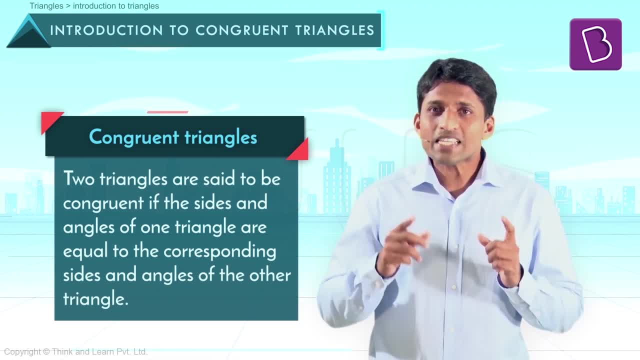 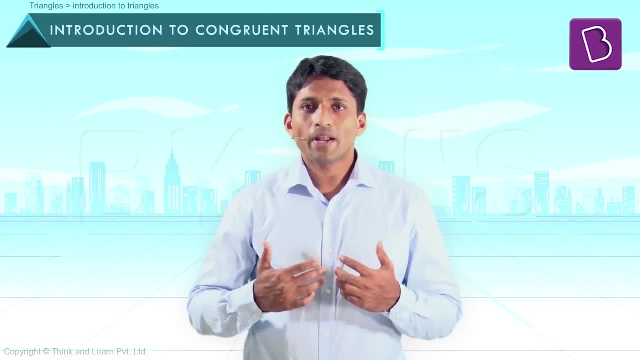 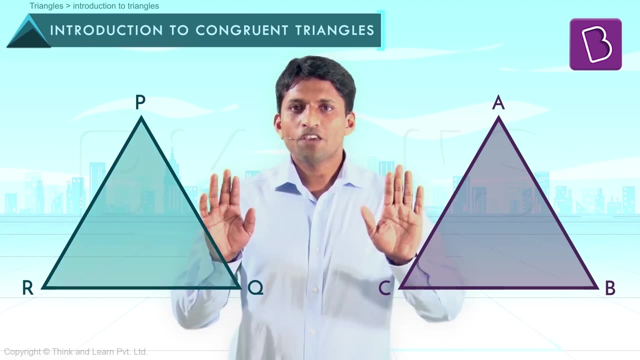 triangle are equal to the corresponding sides and angles of the other triangle. This is going to become much simpler when we learn through diagrams, So let's visualize this. Take two concruent triangles, ABC and PQ. If you place one on top of the other on the corresponding sides, as you can see, 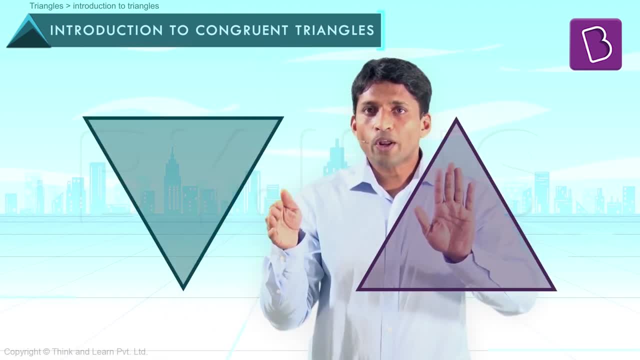 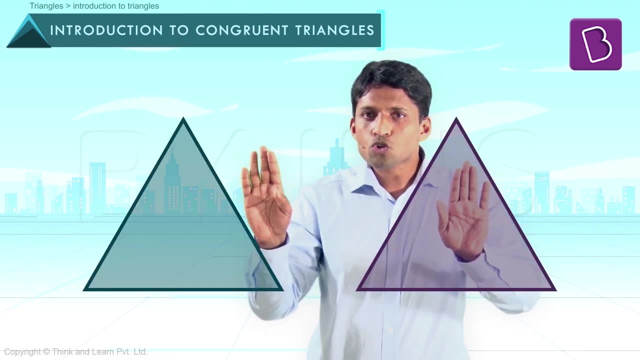 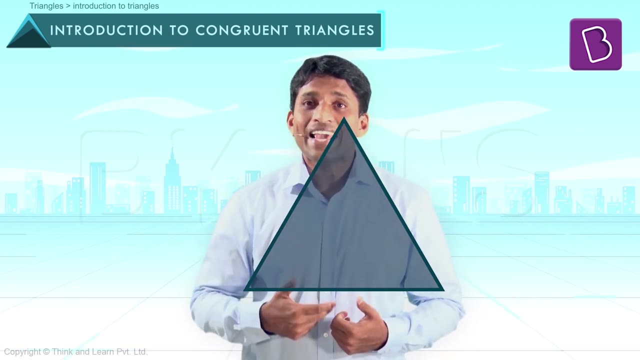 they are fitting exactly Now. you can also rotate, They are concruent. You can flip, They are concruent. You can also slide, and they are still concruent because in all these cases they are fitting exactly. If triangle, ABC and PQ are concruent, this means 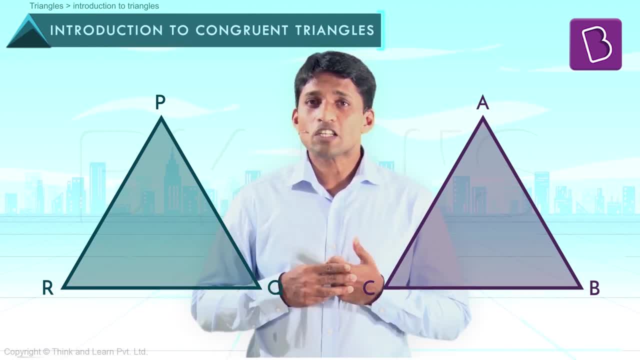 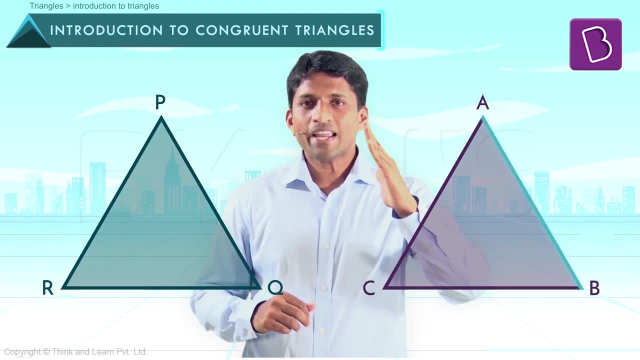 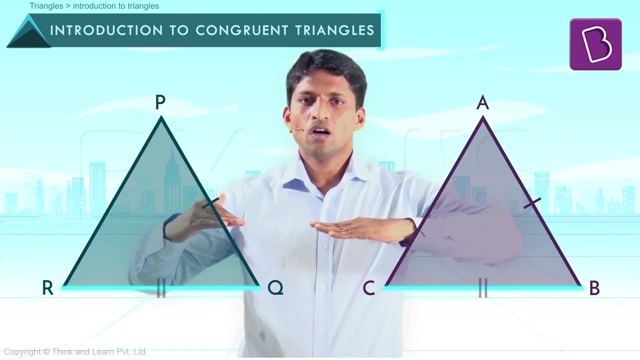 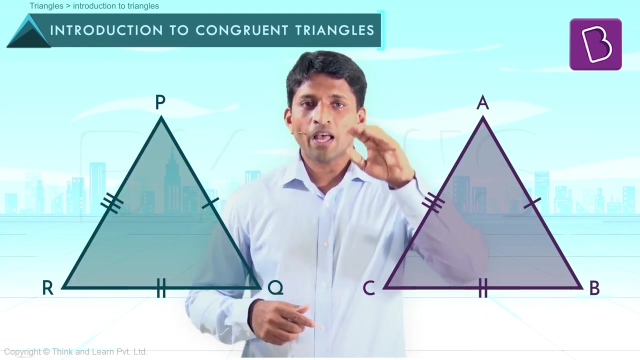 that the corresponding sides are equal and the corresponding angles are equal. That is, in this triangle, ABC and PQ are side, AB equal to PQ, BC equal to QR and AC equal to PR. Same way, the corresponding angles are equal, That is, angle A equal to angle P, angle B equal to. 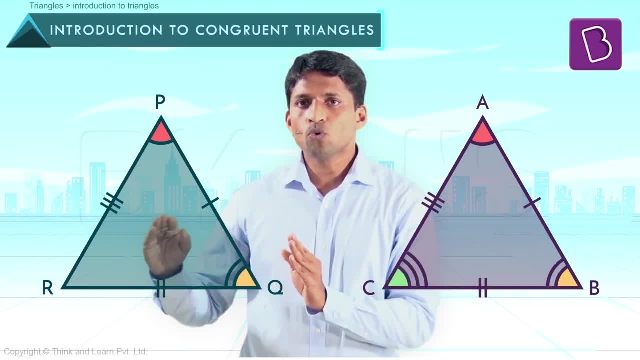 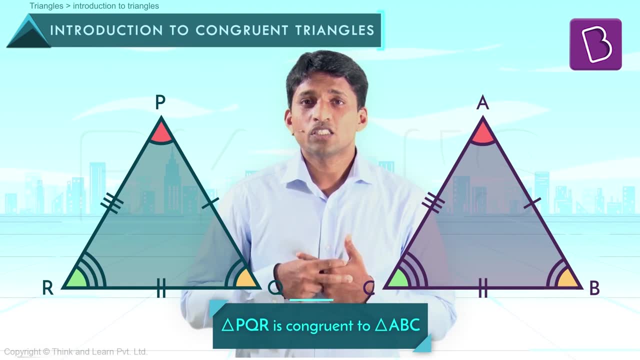 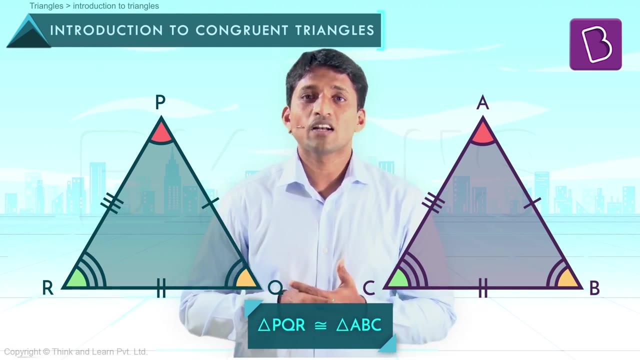 angle Q and angle C equal to angle R. So that's the meaning of concruency: Six parts, that is three sides and three angles will be equal. So there will be three equal pairs of sides and there will be three equal pairs of angles when the triangles are concruent.